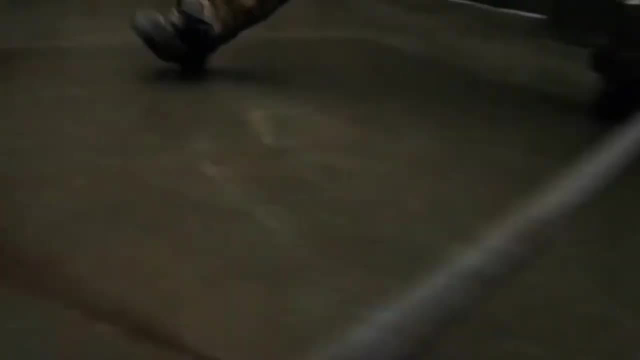 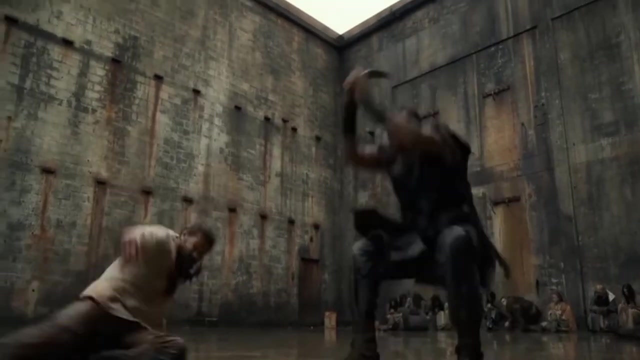 Although the show's $15 million per episode budget may be credited to the show's famous names, such as Jason Momoa, the series' budget is mostly attributable to its Vancouver filming location. To date, the show has been the largest streaming company in the United States. 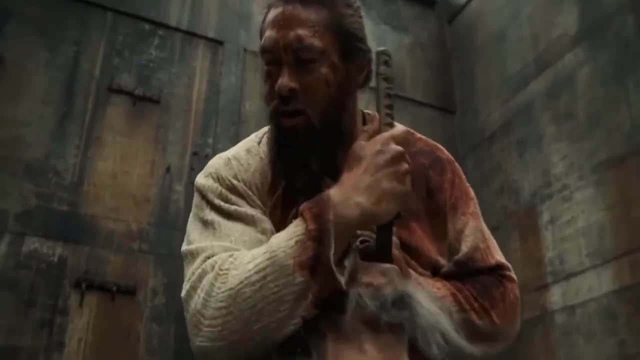 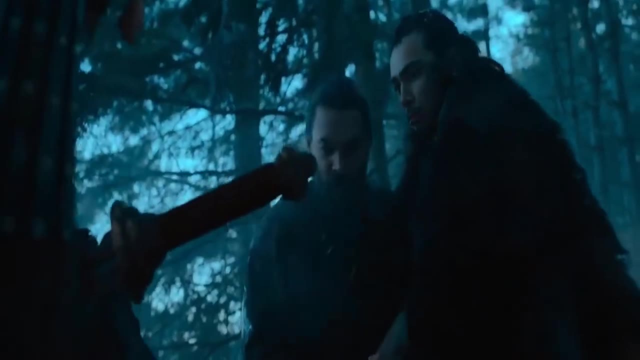 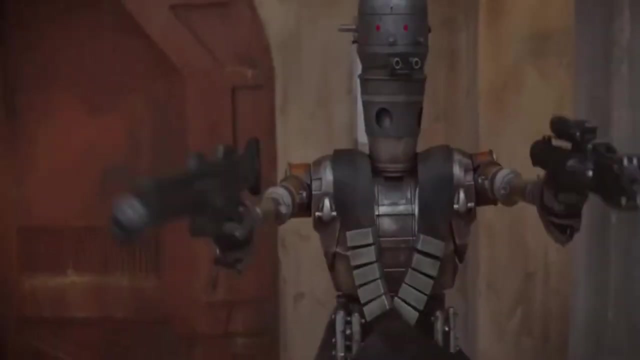 To help create the dystopian environment, the production team drained an actual lake in Vancouver, created a hamlet and then filled the lake after filming was finished. Number 8, The Mandalorian- $15 million per episode. When The Mandalorian arrived on Disney Plus, it became an instant hit because the series took 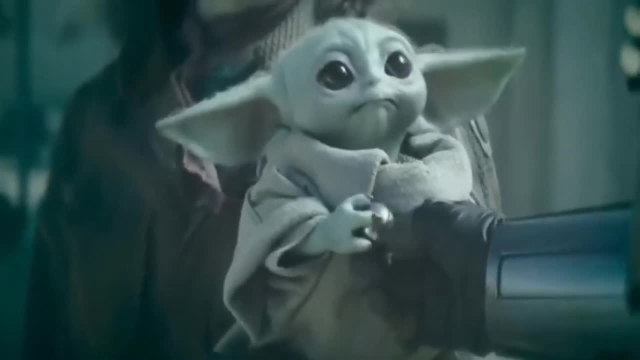 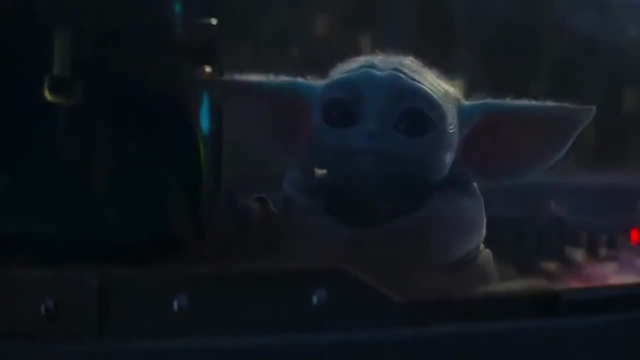 place in the Star Wars world but was not directly tied to any of the major films, It had a lot of leeway in terms of plot and character development. Critics complimented the performers' actions and performances, especially Baby Yoda, who went popular on the internet. 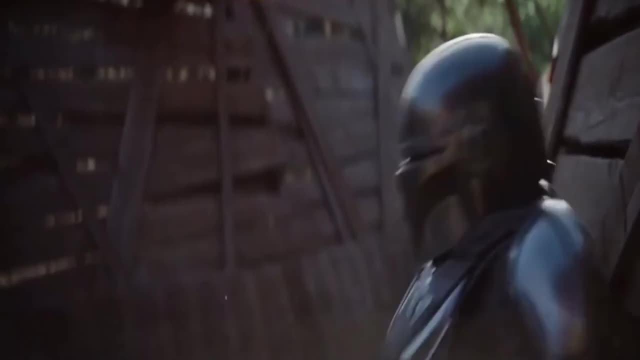 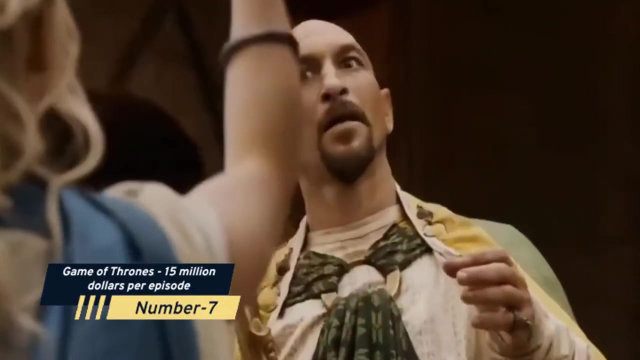 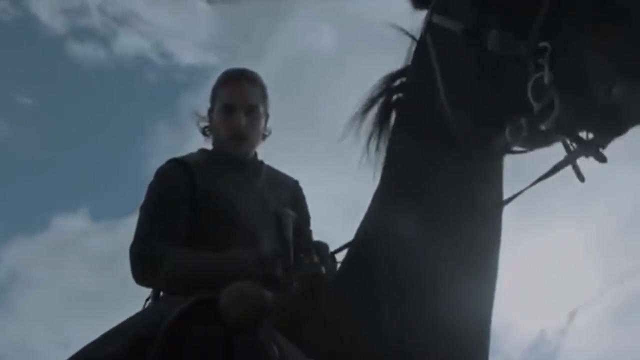 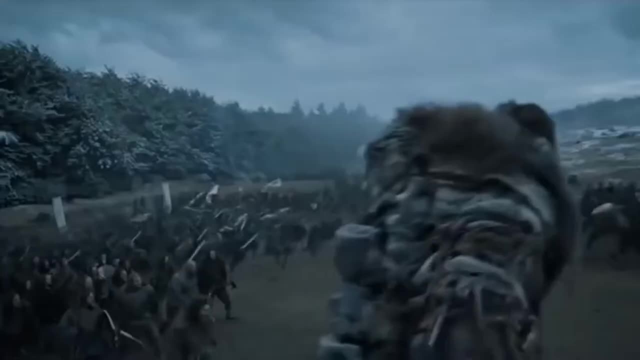 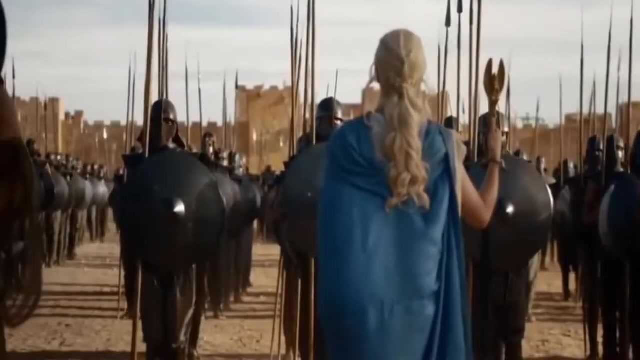 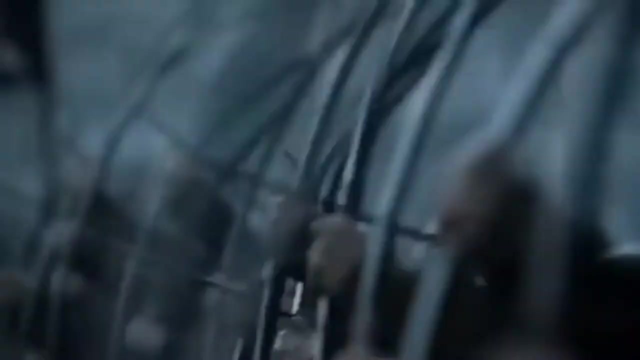 most popular shows in television history came at a high price, for $100,000.. With a gigantic regular cast, thousands of extras, a throne made of real swords, difficult to access, visually gorgeous filming locations and three very realistic dragons, it's no surprise that a large budget 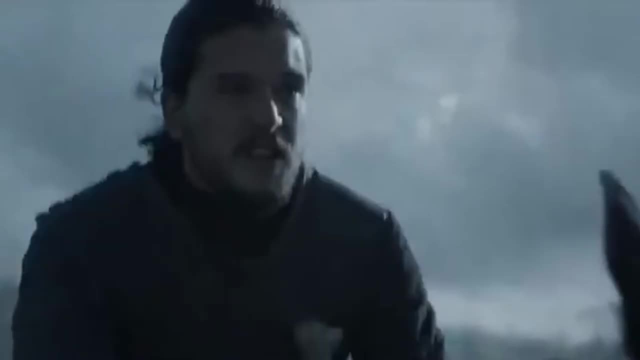 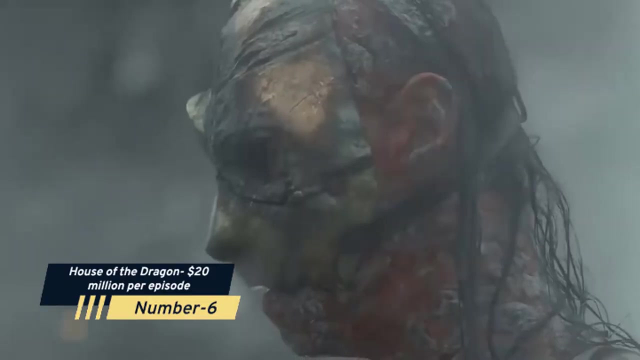 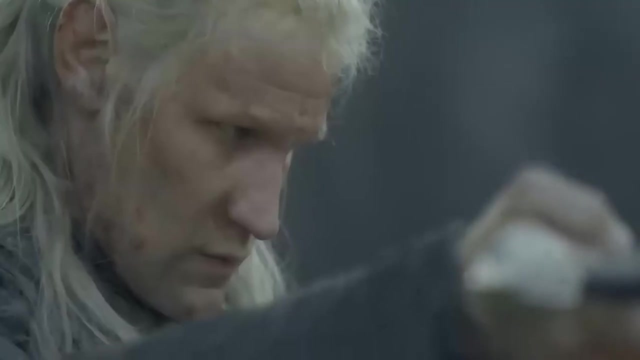 was required to bring GRR Martin's books to life. The last season was the most expensive to create out of the eight: Number 6.. House of House of the Dragon: $20 million per episode. The series is set two centuries before the events of 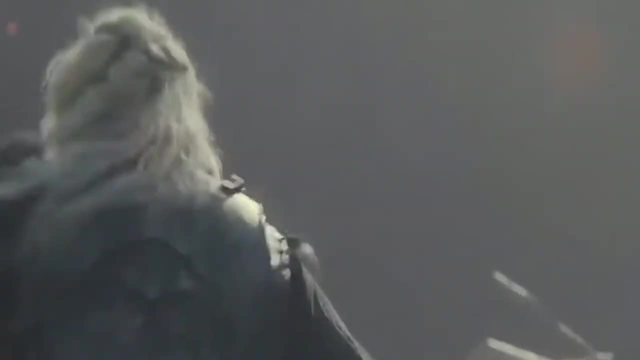 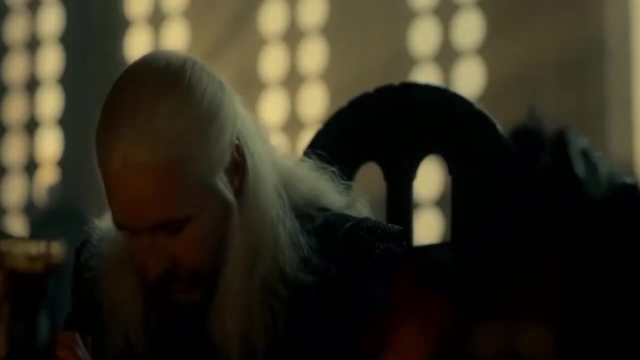 Game of Thrones and focused on the House of Targaryen and the civil war that led to the family's downfall and the departure of dragons from Westeros. building on the popularity of its predecessor with 10 million views in the first episode, With lots more CGI dragons and 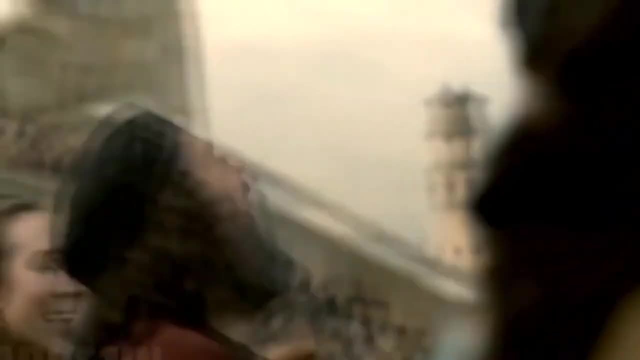 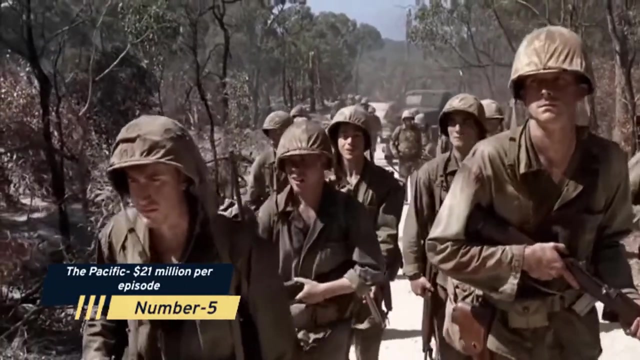 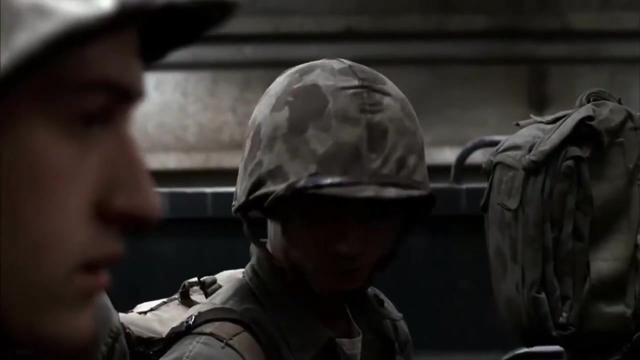 predicted success of a Game of Thrones prequel. the $20 million per episode budget has allowed the series to deepen the story of Westeros. Number 5. The Pacific: $21 million per episode. The Pacific based on the historical events of World War II, combat between Japanese and. 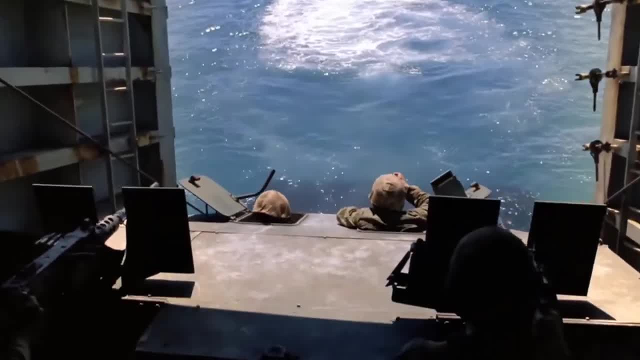 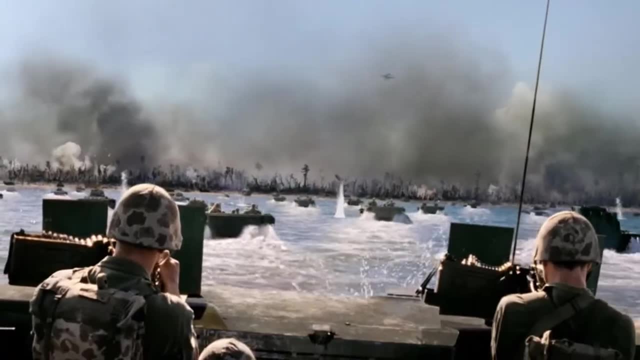 American soldiers on the island of Peleliu was the costliest miniseries at the time, At $20 to $21 million each episode. the HBO miniseries received critical acclaim for its historical accuracy and depiction of epic World War II Pacific Ocean. 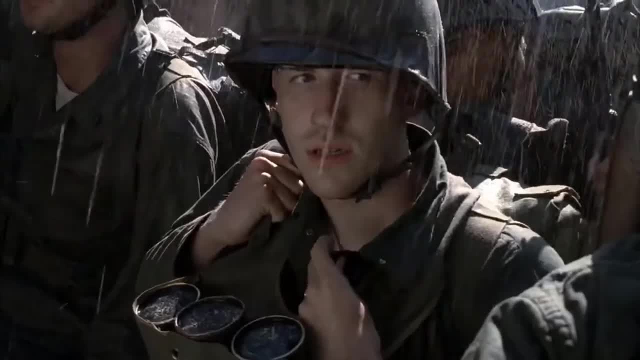 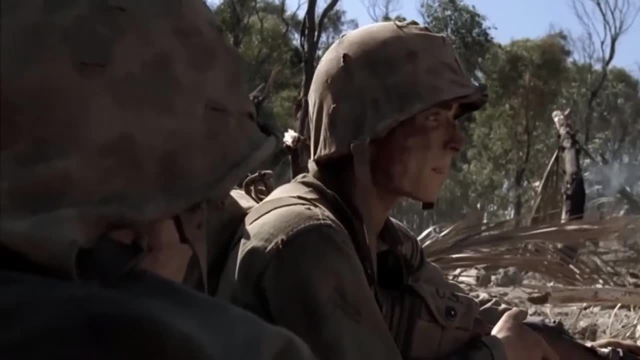 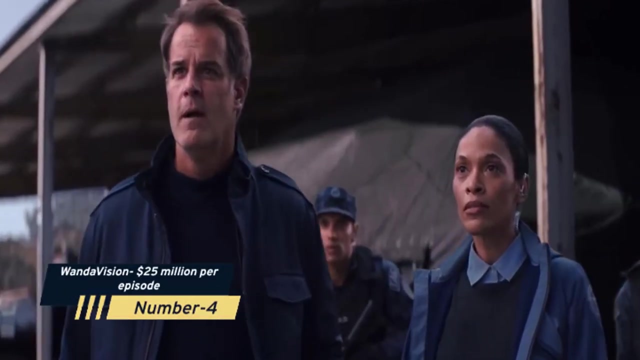 battle scenes With huge names like Spielberg and Tom Hanks. behind the production and legendary film composer Hans Zimmer. behind the military drama score, the Pacific feels like a TV program on a grand cinematic scale, Number 4.. WandaVision: $25 million per episode. 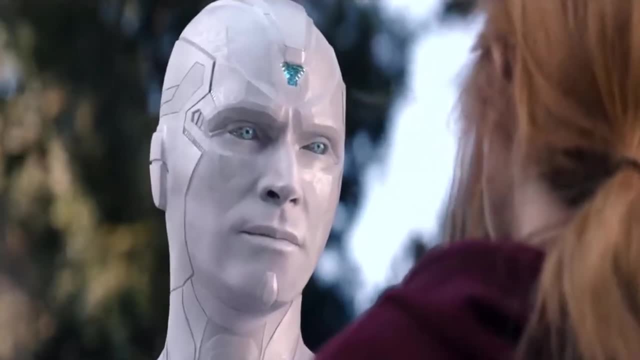 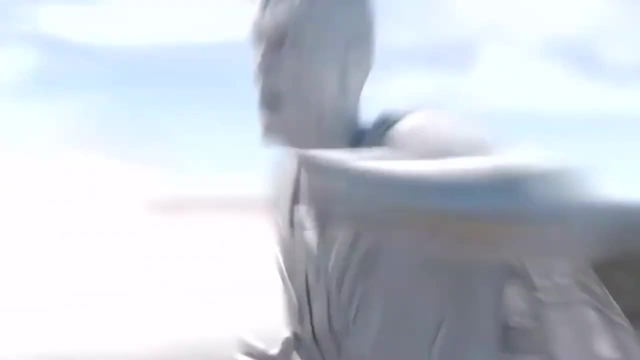 With a $400 million per episode. the HBO miniseries received critical acclaim for its historical accuracy and depiction of epic World War II combat between Japanese soldiers on the island of Peleliu. Marvel's foray into television following the dramatic finale to the Infinity Saga was accompanied. 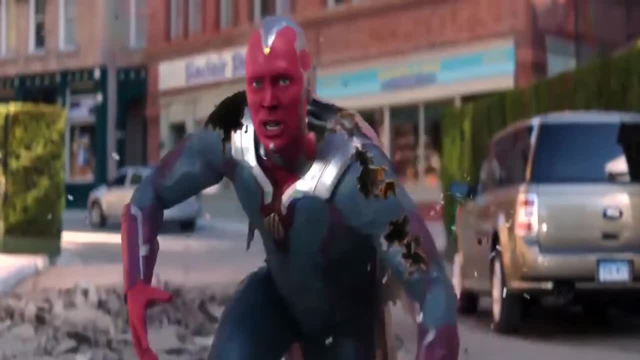 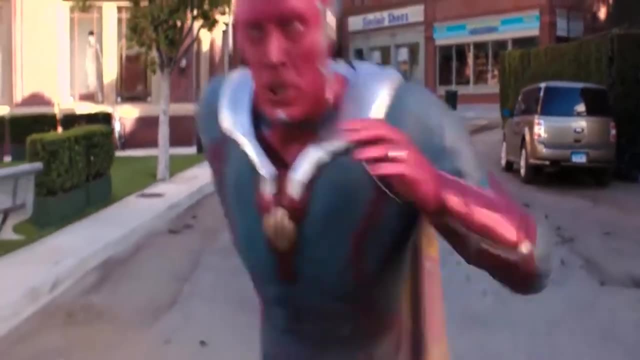 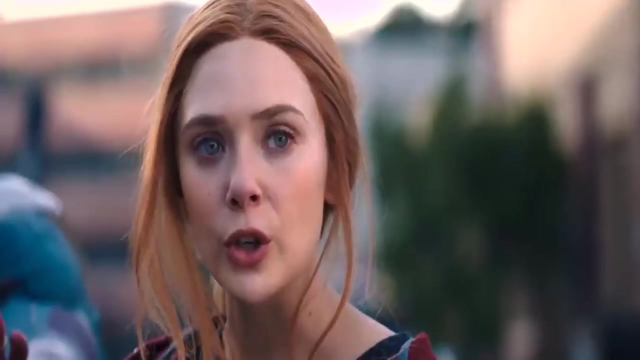 by similarly large expenditures to continue developing the MCU. Marvel paid $25 million per episode after the introduction of Disney Plus in 2019, on each of their new MCU television properties: WandaVision, The Falcon and the Winter Soldier, Loki and Hawkeye. 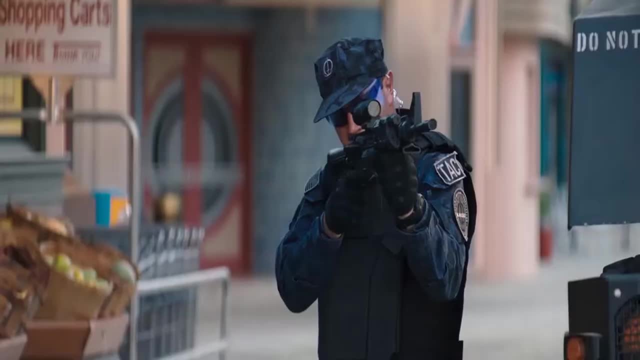 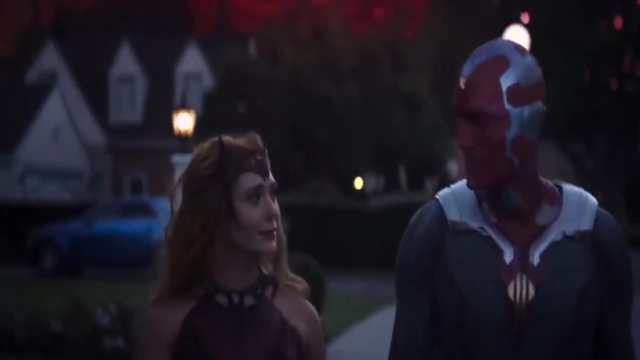 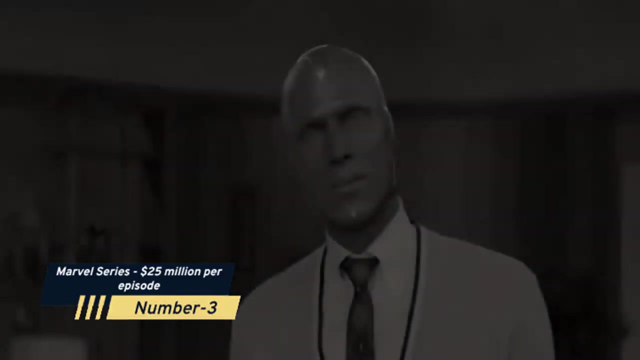 Soldier Loki and Hawkeye. With the release of She-Hulk, Attorney at Law, and a consistent influx of content throughout the year, it's evident that Marvel is dominating both the big and small screens. Number 3. Marvel Series. Disney Plus is focusing all of its efforts. 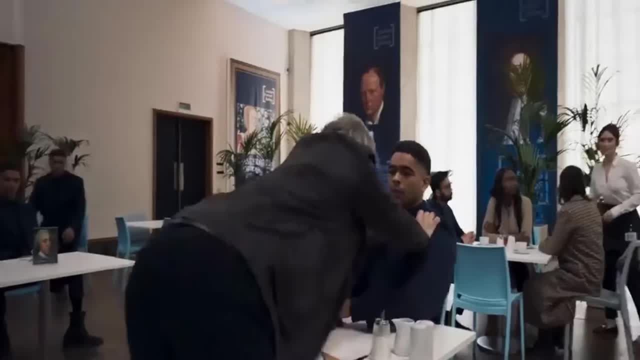 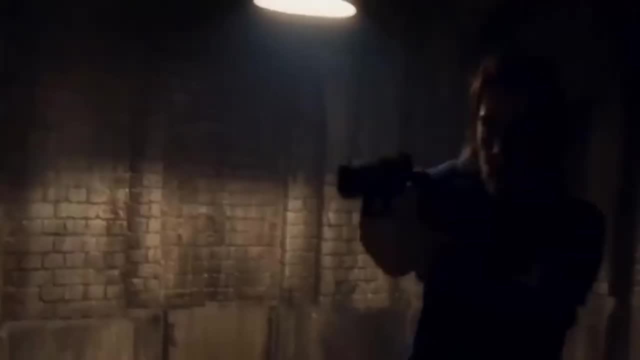 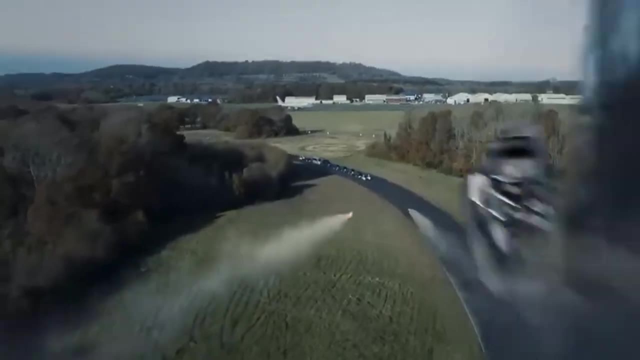 on streaming and with its flagship MCU seeing amazing success, It's easy to understand why There are now multiple shows available, with a long line waiting to be released, with shows like Loki The Falcon, The Winter Soldier, WandaVision and Hawkeye.